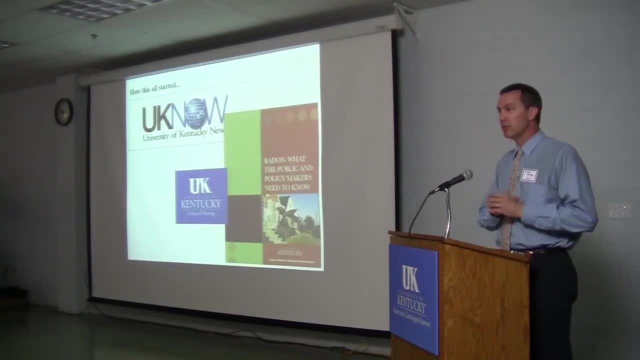 For those of you that are on campus, you know that we get these frequent emails from something called UK NOW or You Know, depending on how you want to read the acronym, And it's just this sort of regular update of campus news about different awards, faculty have gotten different projects going on, different events that the UKPR people want to highlight. 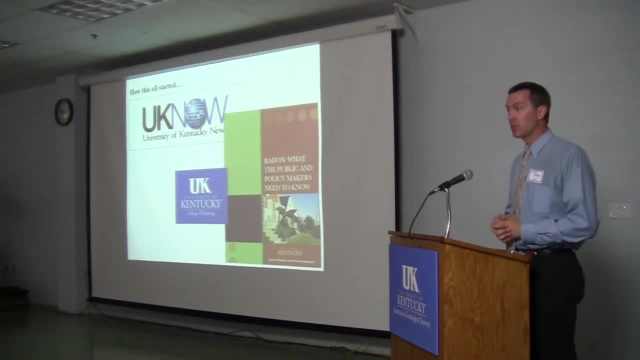 One of these articles about two years ago that Skrull passed was was about the College of Nursing doing some work on radon And they had produced a new publication on what public policy makers need to know. We thought this was interesting. 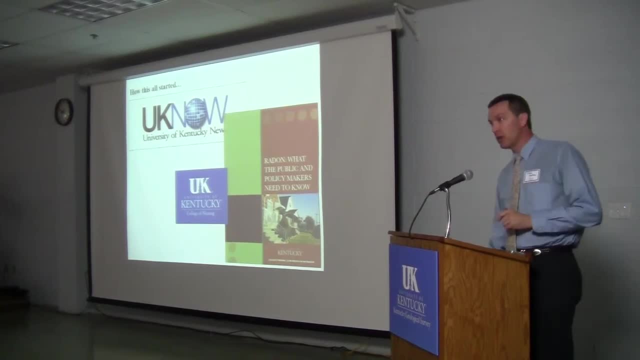 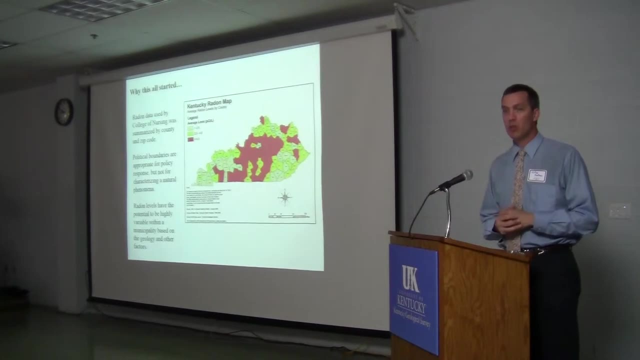 We explored that And we found that a lot of their information was county-based, Which is fine, But as the geologic mapping section, we're very aware that the geology of a county can vary quite widely over short distances, And so 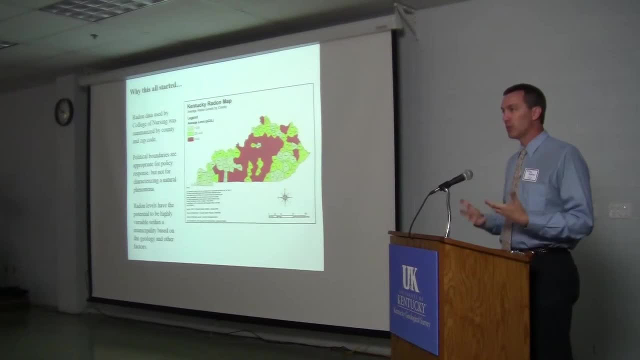 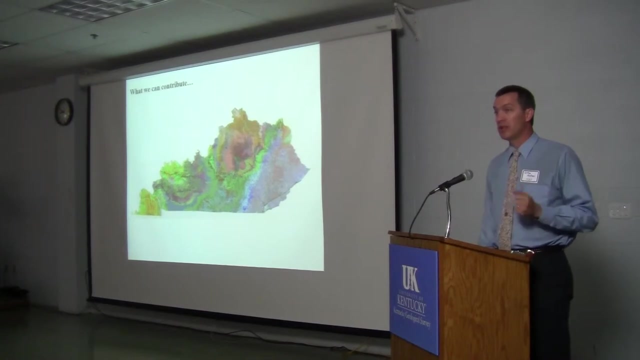 Redline certain counties with. this approach might be unfair to certain homeowners Versus other areas that might not be getting concern in some of the medium counties etc. So we felt like there was a better way to display and illustrate radon potential And we approached the College of Nursing with our geologic maps. 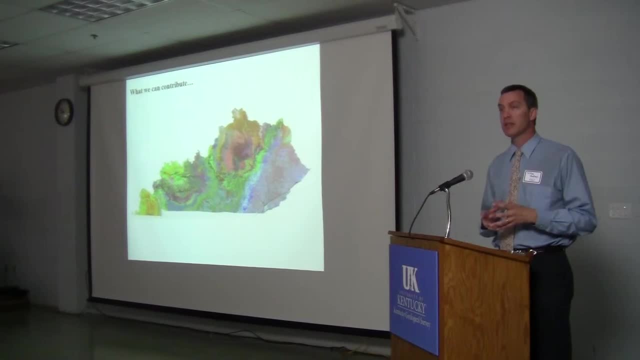 And this turned out to be one of the more challenging parts of the whole process- Giving non-geologists non-scientists. Well, they're not non-scientists: They're health scientists. They're not spatial scientists, The way biologists and geologists are. 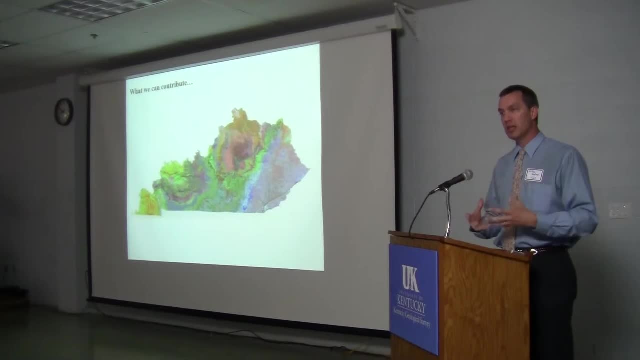 And to get them to appreciate what a geologic map represents. The complexities, the sophisticated portrayal of earth materials is not something they had a background to really appreciate. But they listened And they got it. We started with a county demonstration. They had done a recent project where they had collected a lot of radon data in Boyle County. 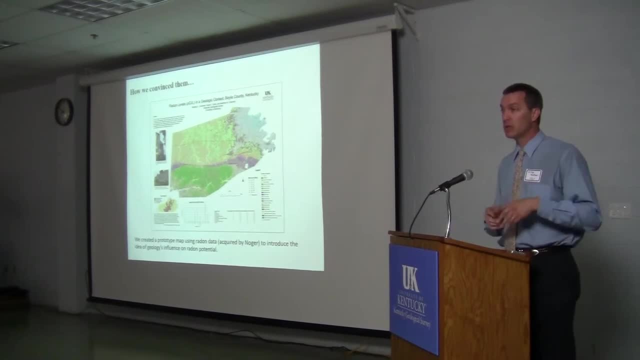 And they already had that information And they shared it with us And we turned around, put it on a geologic map, Gave it back to them, Illustrating how different geologic units had different radon characteristics, based on just their data set. 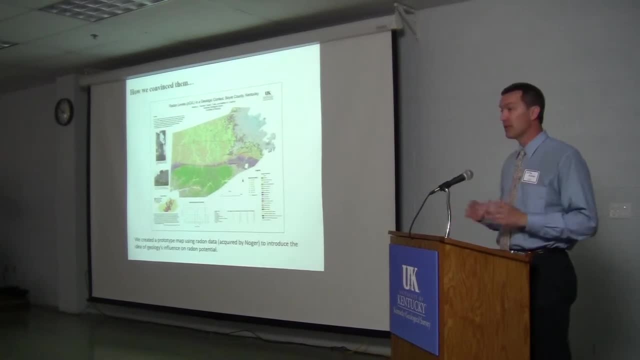 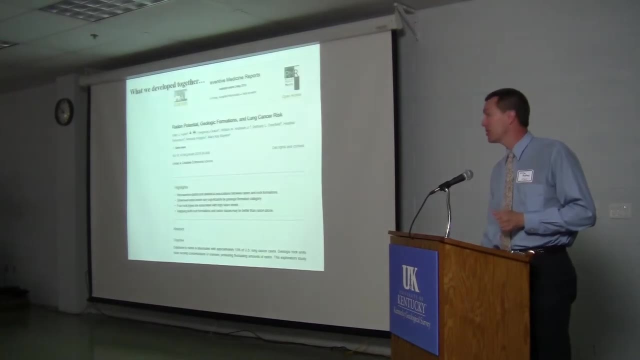 Which was they admitted even a limited data set. This sold them And they went out and got us funding. They went and pursued some funding to do a statistical study on radon potential in geologic formations And how that connects to lung cancer risk. 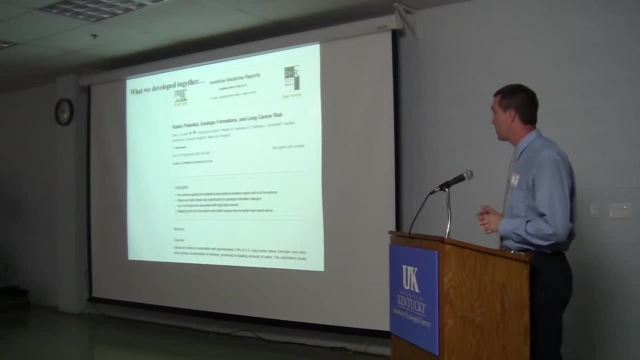 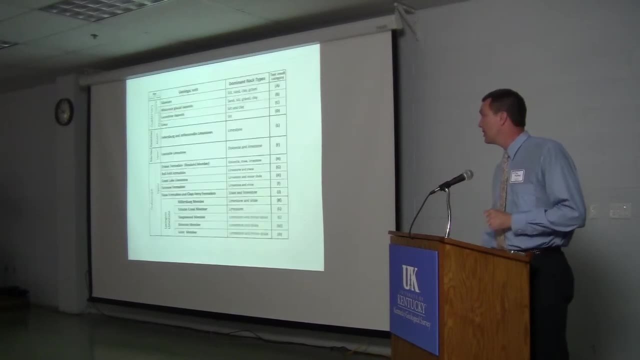 And published this in Journal of Preventive Medicine. This is Citation is almost complete. It's in their online version now, But the basic idea was that we take the stratigraphy. We have detailed geologic mapping with 1 to 24,000. 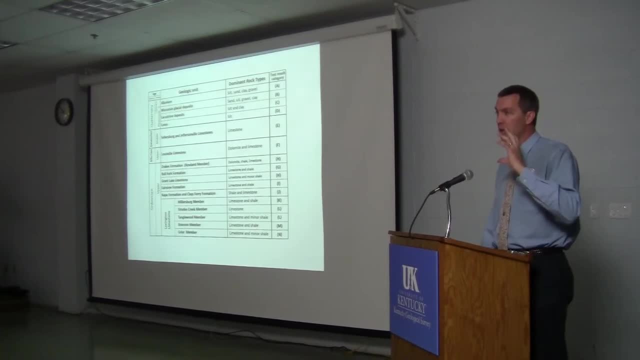 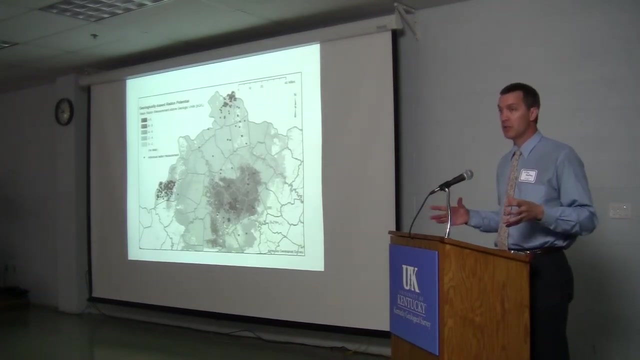 We can take some of those map units and group them together because of their similarities of composition. So we went through a target area And grouped the stratigraphy And looked at the radon locations, Which were not evenly distributed. They were scattered where population centers are. 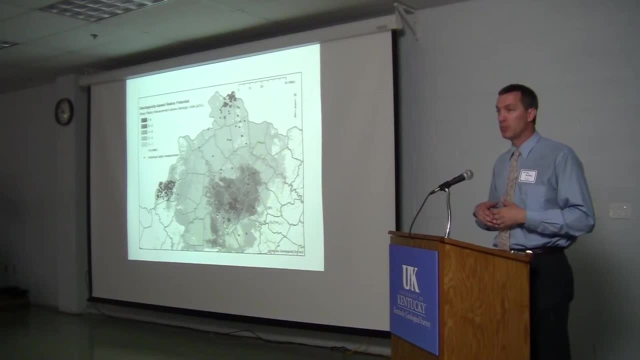 But they were. There were enough points on enough map units that we could say Something. Now this data set came from some information that MC Noder and John Kiefer- I saw John here earlier- They collected this years ago. They connected the body of radon measurements that the state had. 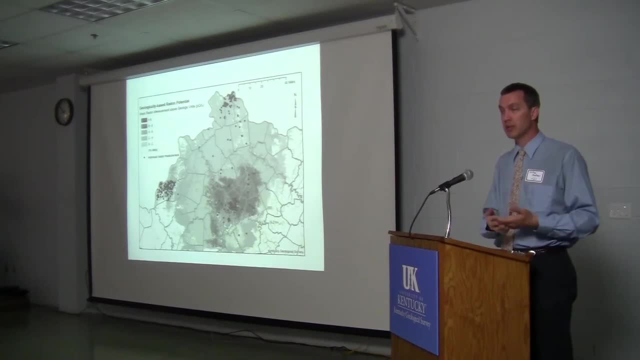 They connected geologic information based on its location And then it just kind of sat there. Nobody did much with it. A couple of years ago Brandon Nuttall got that information digitized And then made a quick map out of it for a question that somebody had sent in. 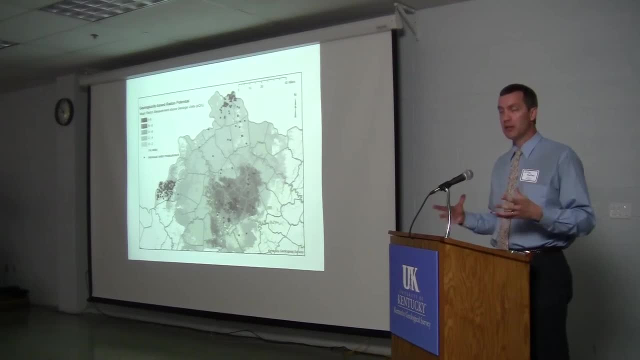 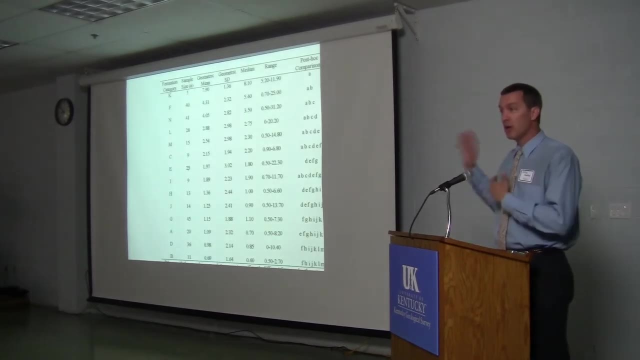 And so that was the data. we had About 900 data points. We used about 300 of those, And what we were able to do is show that. Don't try to understand this. The point is, the statisticians were satisfied And very convinced that there was indeed a statistical reality. 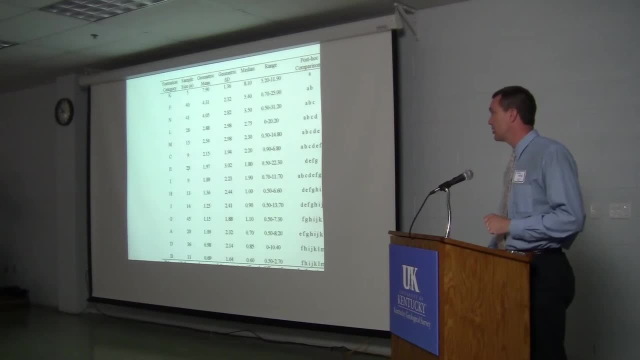 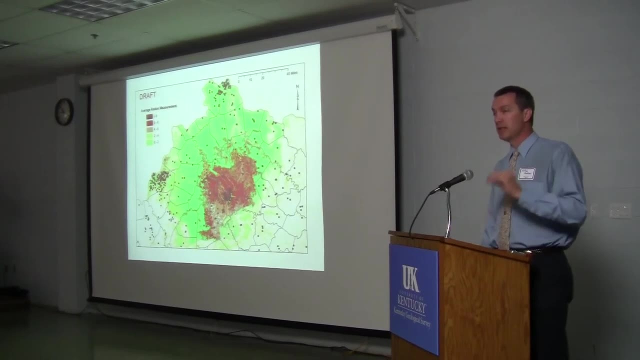 To the variation of the radon Across these geologic units, And so we were able to make A draft radon potential map To illustrate to them That different areas of the state Have a different potential radon risk. This isn't saying this is the absolute radon coming out of the ground. 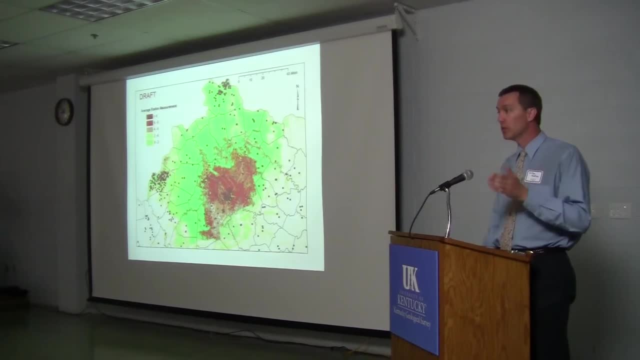 It is saying that these are the areas that have more or less potential for radon. A poorly designed home Can still super concentrate radon in one of these low potential areas, And a well designed home Can have very low radon measurements. 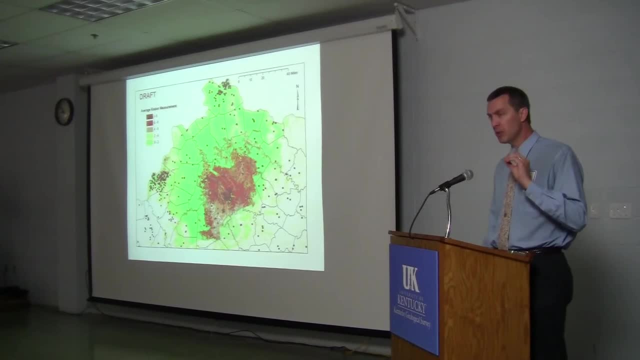 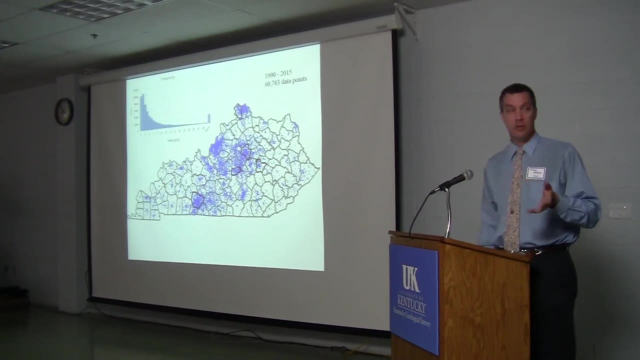 In one of these high potential areas. So the homes itself. The home itself Has a lot to do with the outcome. 300 points doesn't do the job. So again, The College of Nursing people went out On our behalf And got us funding. 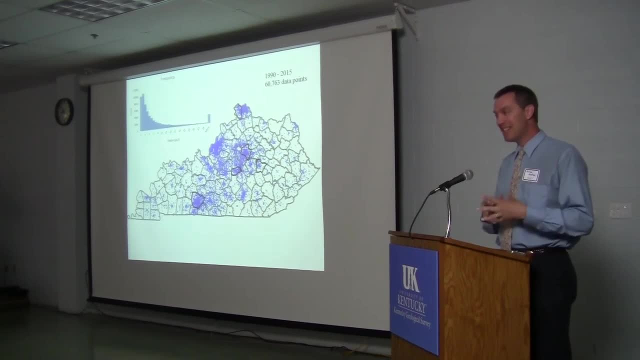 And acquired for us A data set of 60,000 plus Radon In home radon measurements Statewide. We have almost every little geologic polygon In the state Represented here. Again, It is concentrated in the populated areas. 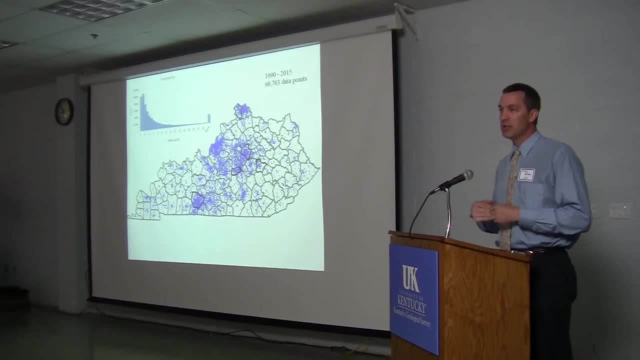 Because that's where the homes are, That's where they're collecting. But when we go to the statisticians And say, do we have enough points On enough of these units, They're quite satisfied with the end values That we get. looking at this, 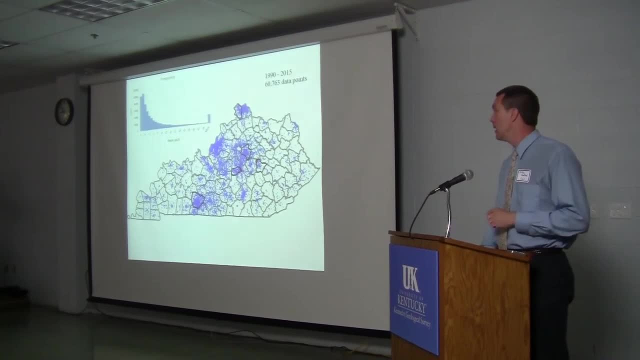 So, going forward, We're going to be making more of these county maps, Like we did the prototype for Boyle County And Boyle and Warren, Using this new data set, The information from this new data set, To make some county scale Radon potential maps. 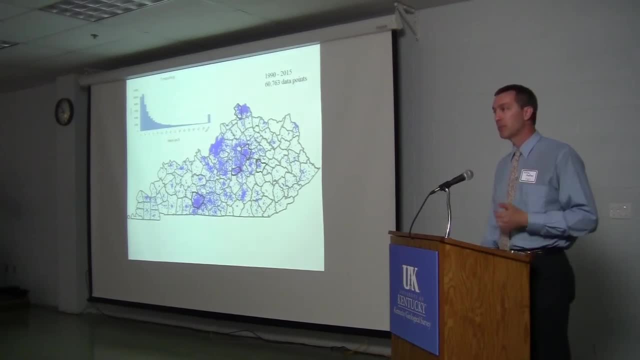 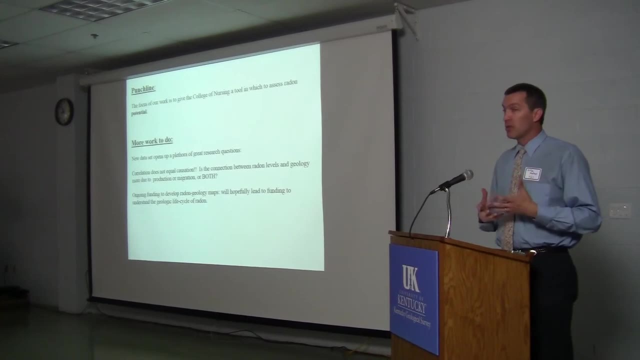 That the local public health people Can then use to target public education And other data collection efforts For their work. So The focus of this project Has been very successful: To get the Public health people to appreciate The geology. 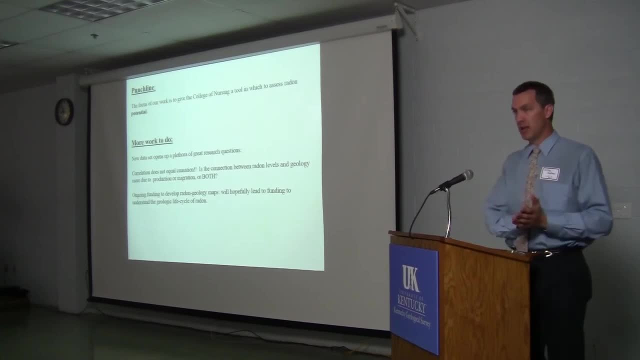 Behind radon potential And that there is a geologic basis for it And not a political boundary basis for it. There's still a lot of work to do, And this opens up Avenues of inquiries For some really good, Detailed, on the ground science. 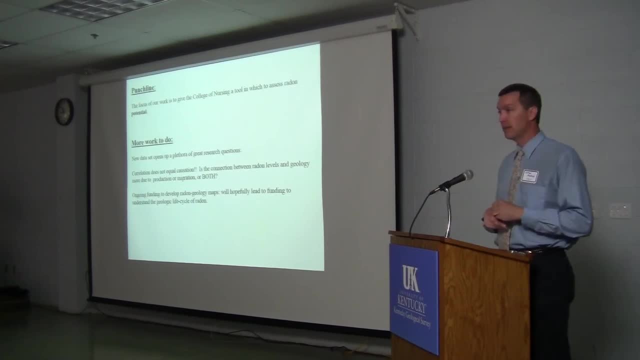 This large data set Gives us a huge opportunity And it opens some questions. Some areas of the state Where we have no preconceived notion Of a high uranium Mineralogy in the rock units Test high for radon, Which then leads us to believe.